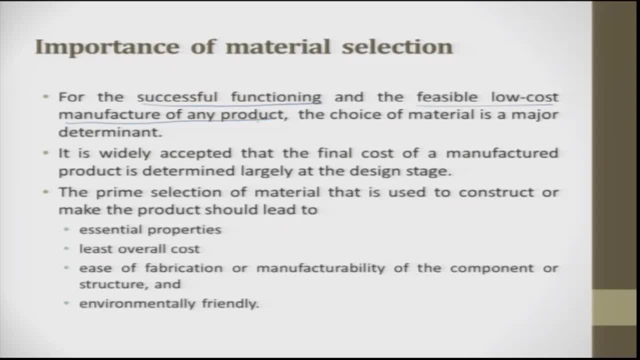 and the feasible low cost manufacturing of any product. the choice of materials will be'll try to cover in our lecture. material is important. A simple example is your chair. initially these chairs were made out of wood, then it changed into steel and today it is all made out of plastics. 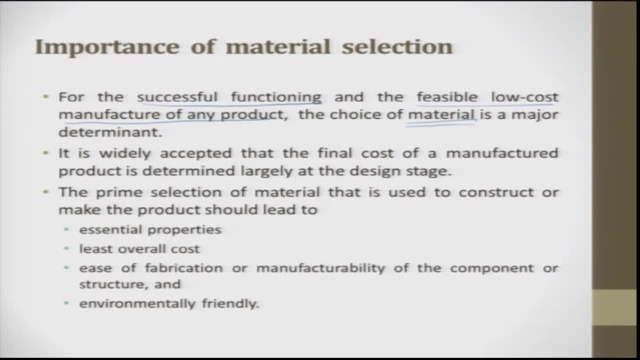 Initially the customer could not digest- how can I sit on a plastic chair? but the product designers presented the chair in such a nice fashion. they brought in lot amount of comfort in the chair. plus they try to have maximum strength, which got integrated into the chair. 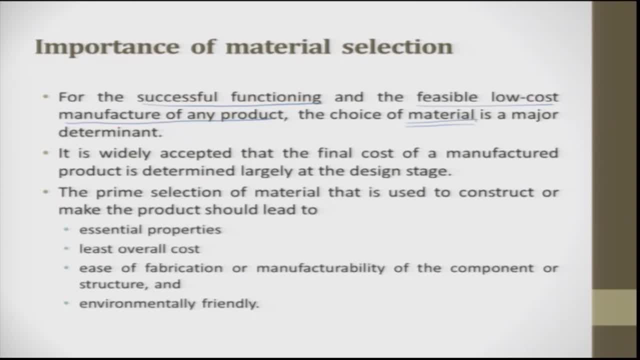 The design of the chair was very wonderful. so this: slowly, slowly, over a period of time, plastic chairs have got accepted by people and today plastic chairs are the most common thing you find in any living room or dining hall in any house. So it is the material which changed from, it is properties, from a soft material to a 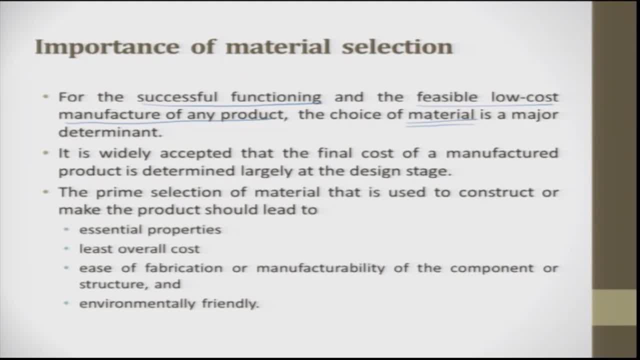 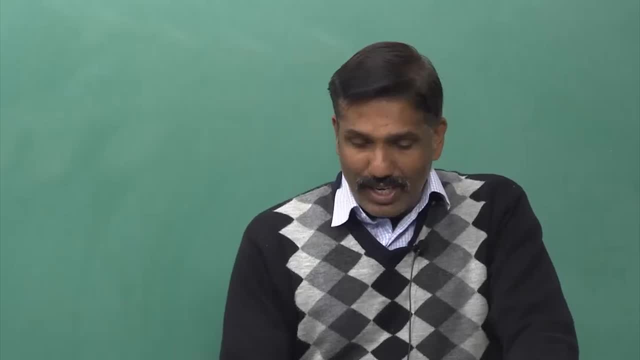 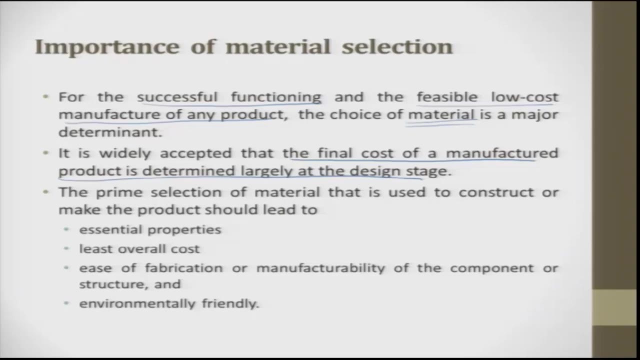 very hard material and a design which is integrated into the material made it a robust structure for people to sit on it. It is widely accepted that the final cost of the manufactured product is largely determined at the design stage. So here it. this point clearly states that the designer- product designer- has to have 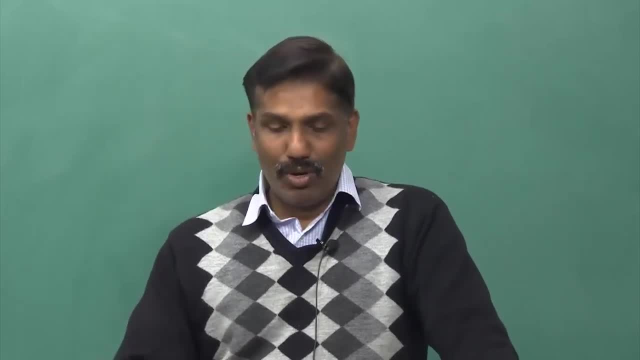 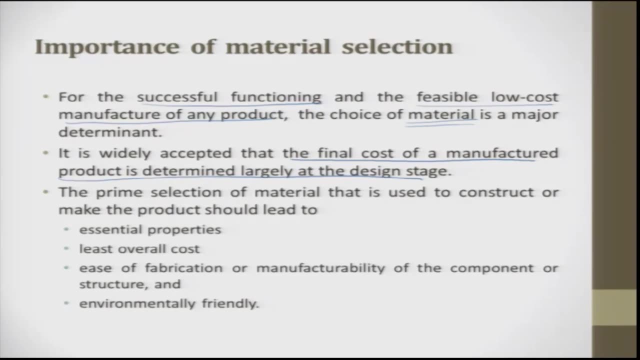 an idea or has to have a team member who is in material expert in his team- The team- to make a proper choice of material and manufacturing. you make a wonderful product but if it could not be manufactured then the product fails miserably. So it is always good to have a materials expert in the design stage itself and try. 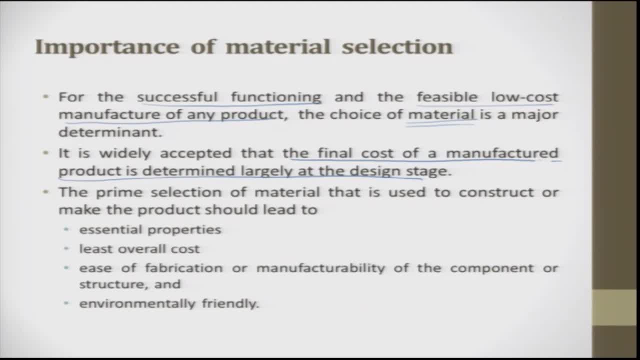 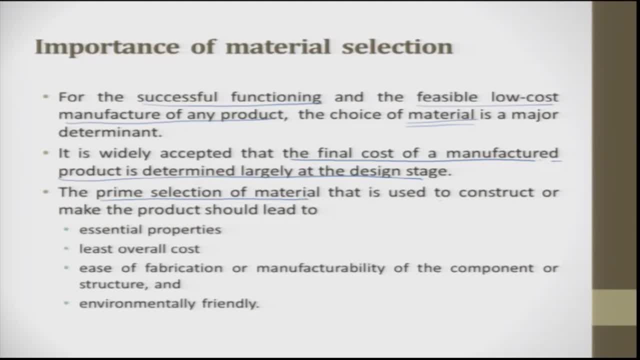 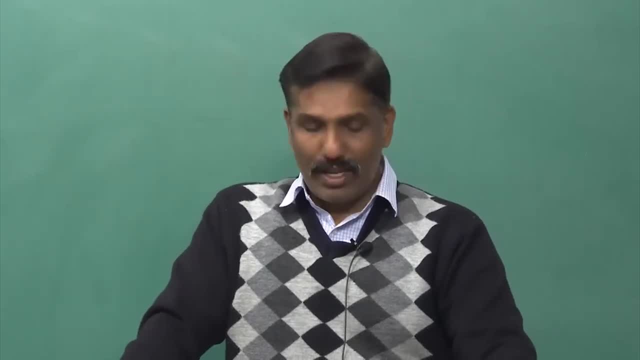 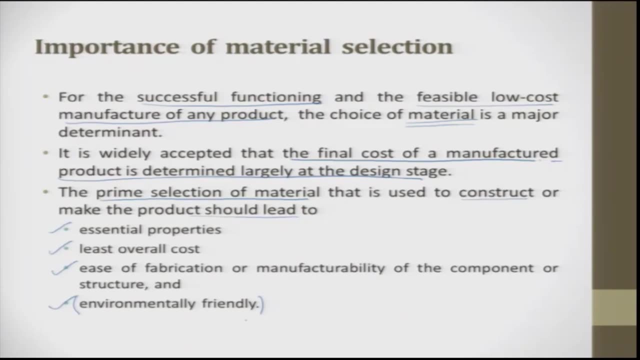 in the products or sustainable materials. So this environmental friendliness is also talked up in a big way. so plastic bags, for example, slowly are getting removed or processing is done such that the plastic can be modified or reused into a different product. So you have to have a proper for selecting a material. you should essentially know its. 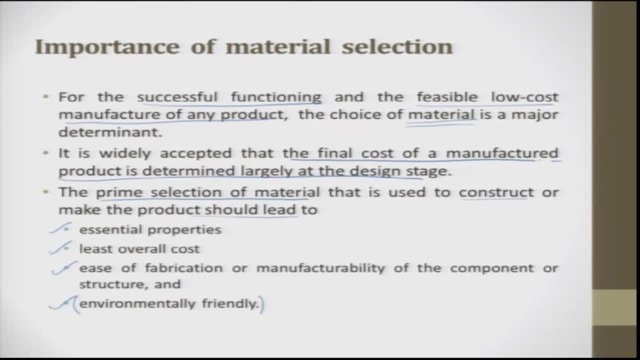 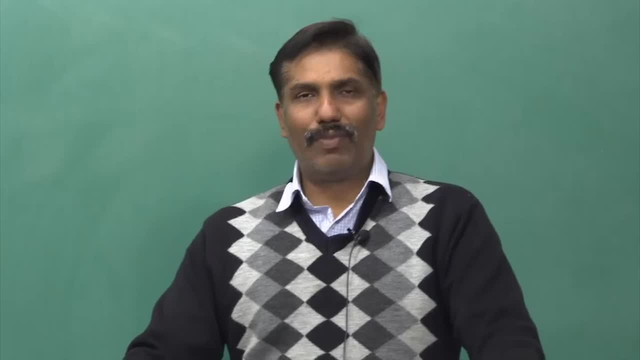 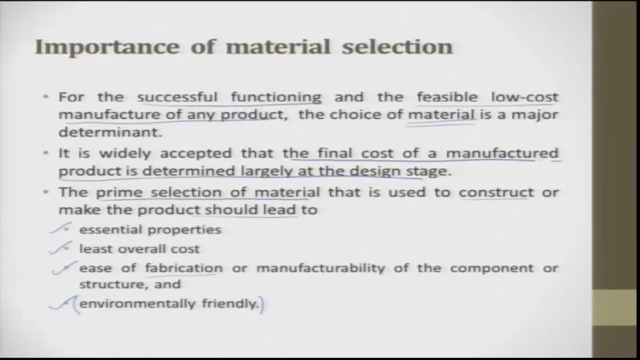 properties and it has to have a least cost and it has to have a ease in manufacturing. Ease in manufacturing is very, very important. For example, plastic parts are very economical because it is one shot process, so the fabrication is very easy, Whereas when you take a steel it is multiple steps have to be done to manufacture and make. 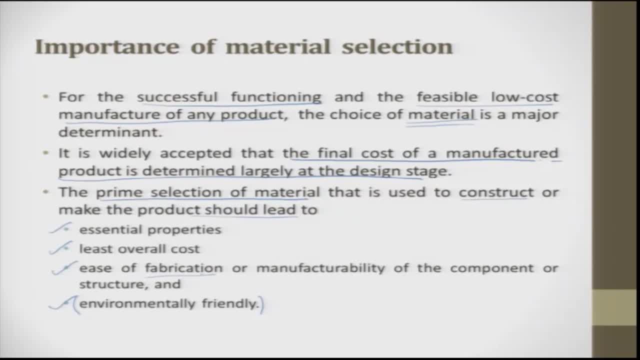 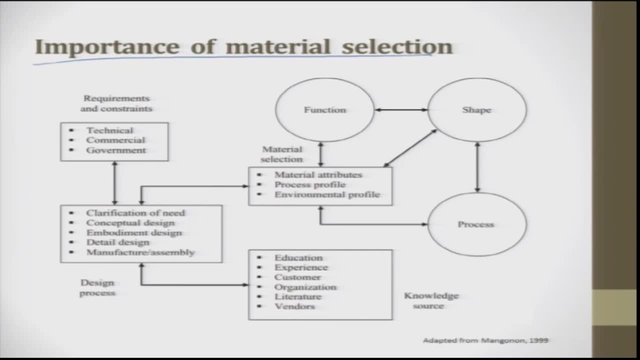 a product. So this is what ease for fabrication. So these are the prime selection for the material construction we have. So when we talk about importance of material selection, shape is very important. shape and size is very important. shape means goes to form. then there is a link between function. 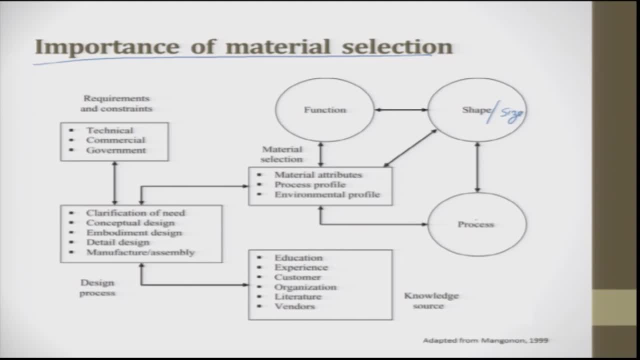 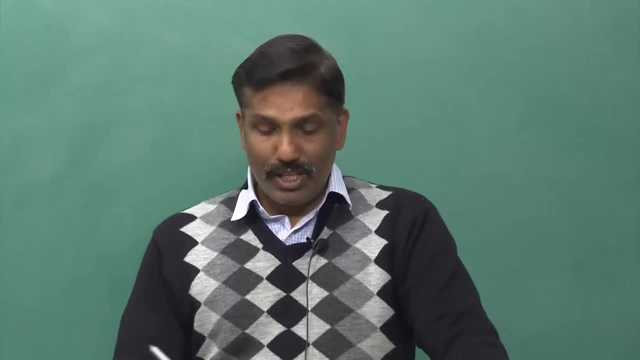 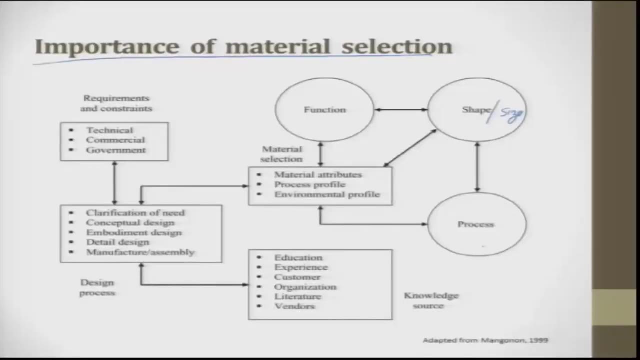 and then there is a link from the shape to the process, Shape and size to the process. you change the dimensions. if you go larger and larger and larger in your dimensions, the process which is involved in making those large dimension products are going to be offered through a different process. so process and then here. 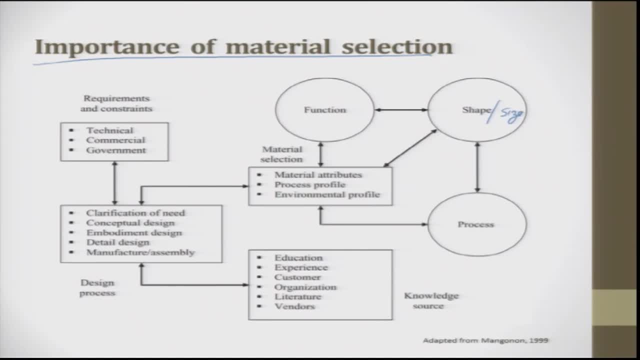 are materials. So the function you have to do, a material selection, which is here, and this in turn is linked, or the properties linked are material attributes, process profiles and environmental profile. So where are you going to use, what is the process to be done? material attributes: how? 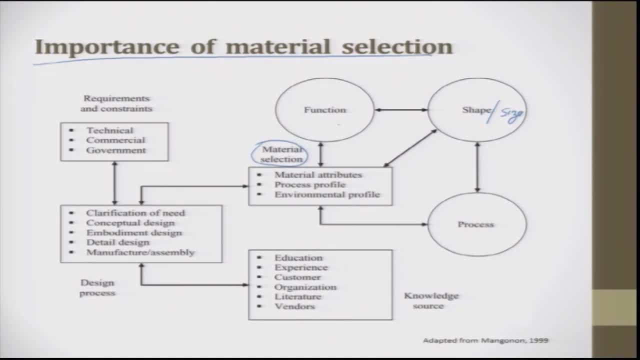 are they? what are they? which is going to make the product very successful? is there? So the function with this? if you try to take this as material selection, they look at these properties and they are linked with the process. So this happens to be back and forth: the functioning processes, shape and size, and 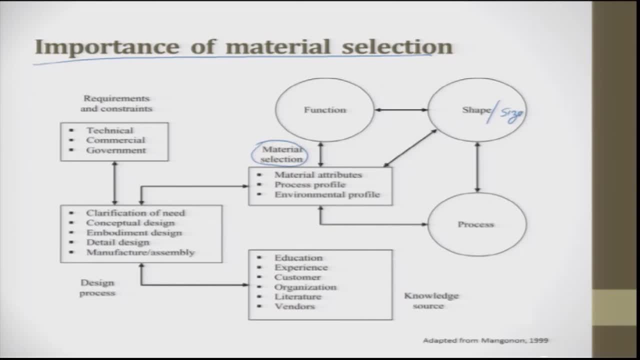 this, all these things go back and forth to get a good product. So the requirements and constraints come from the customers. so you will have technical, you have commercial and you have government constraints, which are there, and then this will lead to classification of clarification of need. conceptual design, embodiment design. 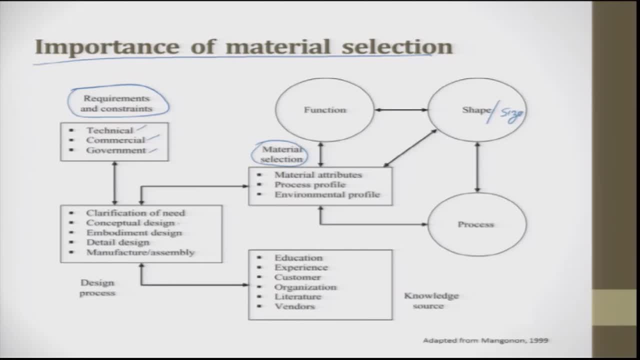 detail design and manufacturing design. they in turn are linked with the material selection or material attributes. So this one is again a back and forth motion. So these are the typical steps which are involved in designing. so, if you try to look, 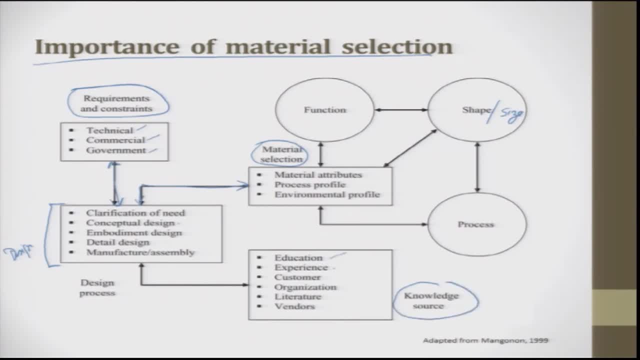 at the knowledge source. where do they get from education, experience, customer organization, literature and vendor? So it is nothing but the voice of the customer, which we discussed in the QFD. so this is what it is. So these are put together. this entire schematic diagram integrates function, shape, size, process. 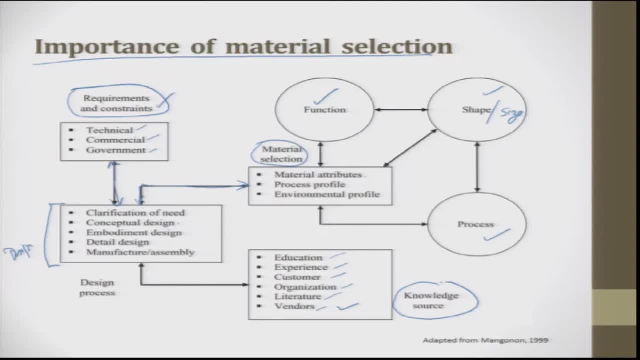 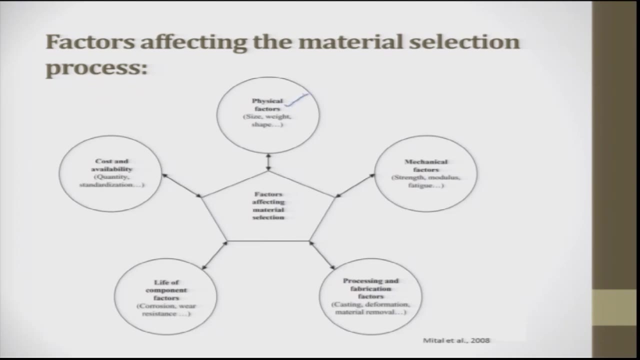 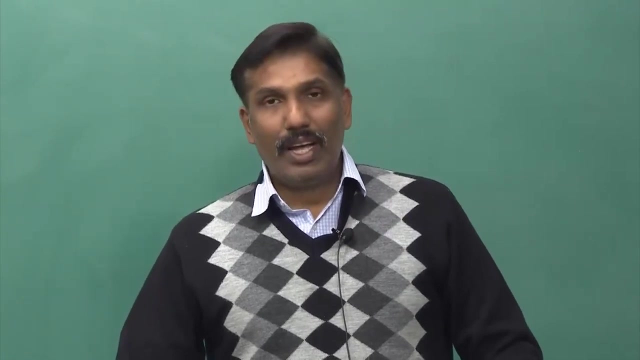 knowledge And the constraints with the material selection. so all these things put together are very important when you try to choose a material. So the factors affecting the material selection process, one is physical form: size, weight, shape. Today we look at: expect a product to be as light as possible, and then we also look at 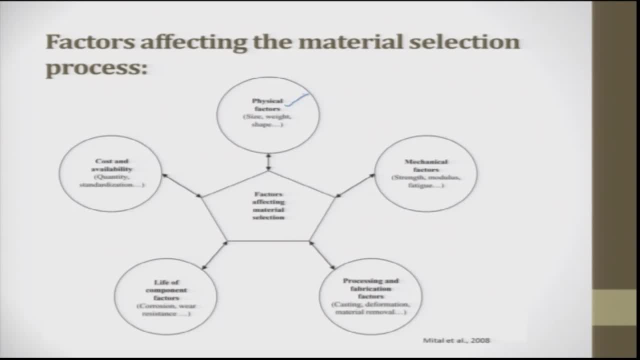 a product which has more comfort. that means to say more customized, So the shape has to be very smooth and it is sleek. they are looking at shapes which are very elegant. weight which is as light as possible, and we also look at products which 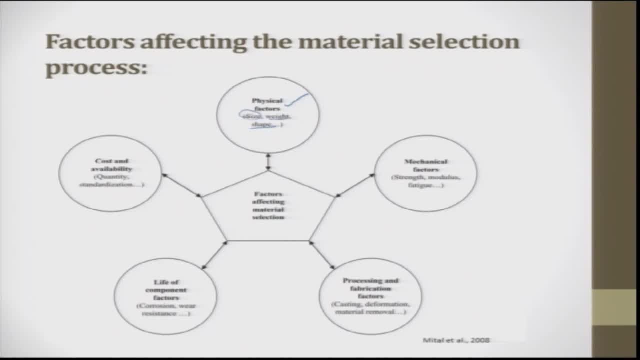 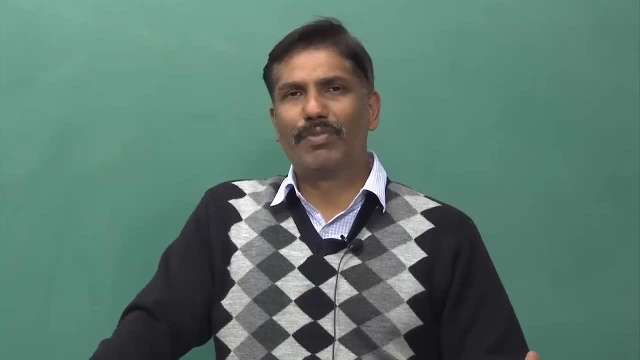 are size as small as possible, for example cell phones. the sizes have gone down. The first cordless phone which came into the market had was at around the weight of 1.5 kilos. Today we talk about a cell phone of 100 grams or less than 100 grams. 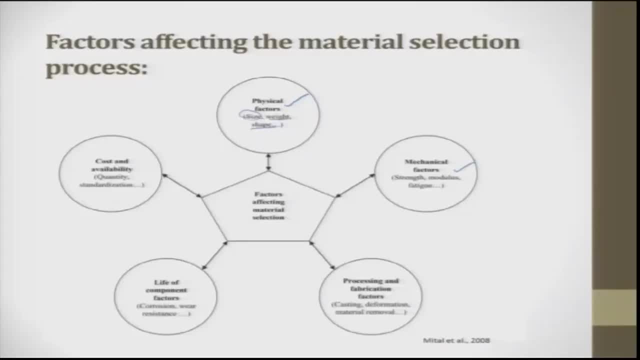 So then this one, the mechanical factor, is the other thing where in which we talk about the strength, modulus and fatigue. So the strength modulus: strength is talked about in the plastic region, modulus is talked about in the elastic region. fatigue is nothing but cyclic loading happening on the, on the 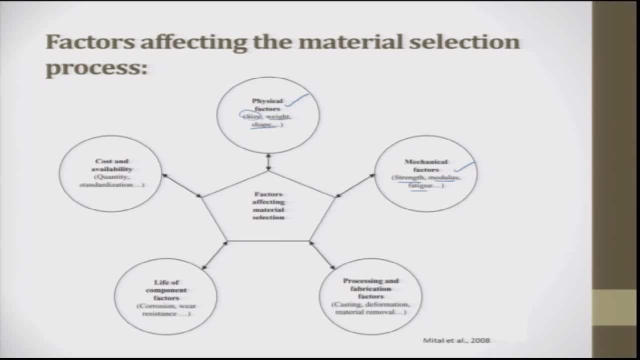 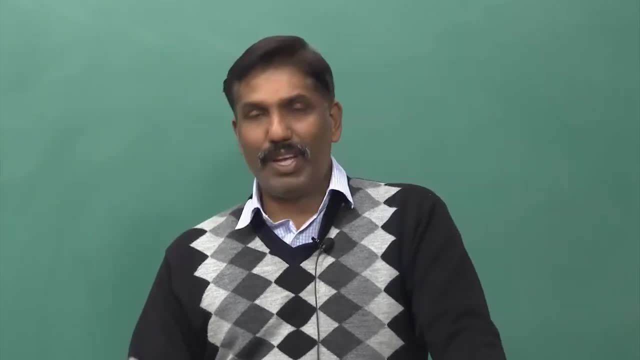 material, if which it has to the product, on the product which it has to withstand for a longer time. So, for example, a chair: chair, when, when a person sits, it is going to be an impact load And then he gets up and then once again he sits or he slides. it is cyclically, it is getting. 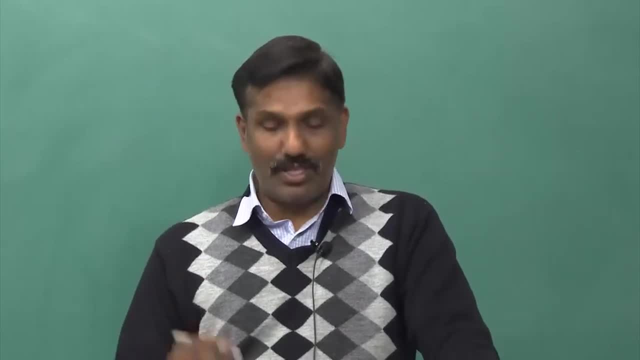 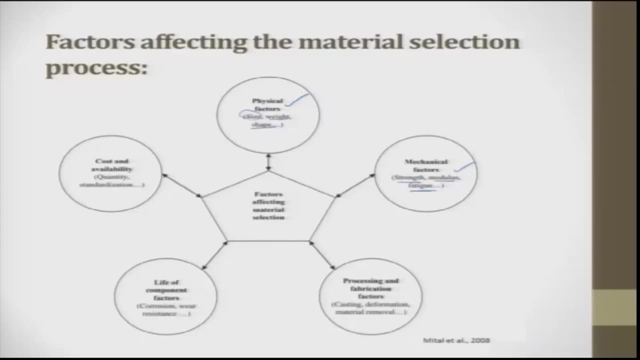 loaded impact load is there. when one person gets up, the other person sits, it is another load which comes in, So it is a compressive load which comes here, so it is fatigue. So all these factors are mechanical factors. So here are size factors. these are mechanical factors. then you will have processing and 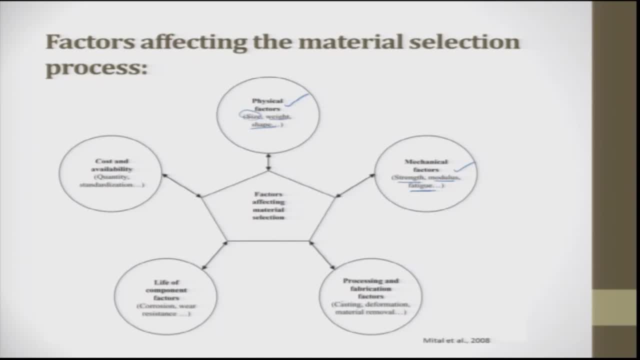 fabrication factors say, for example, whether to be done by casting deformation. casting means you try to take it to a higher temperature, melt it and then pour it into a die. casting Deformation is you apply load and you try to deform a material. it is deformation. and 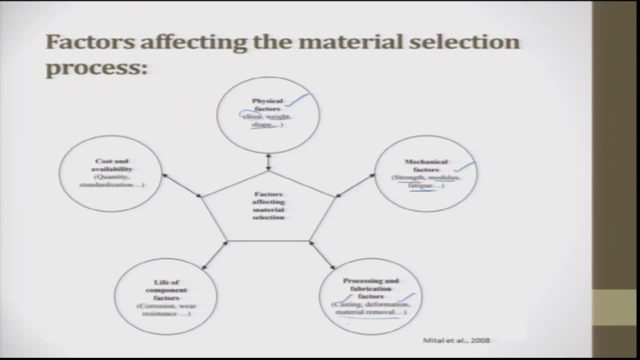 then you have a subtractive process called material removal, where in which this, the unwanted material, are removed and then you get the feature, what you want. So the processing and fabrication factor is also important to decide where the what is the material for the given product, the life of the component and factors like corrosion. 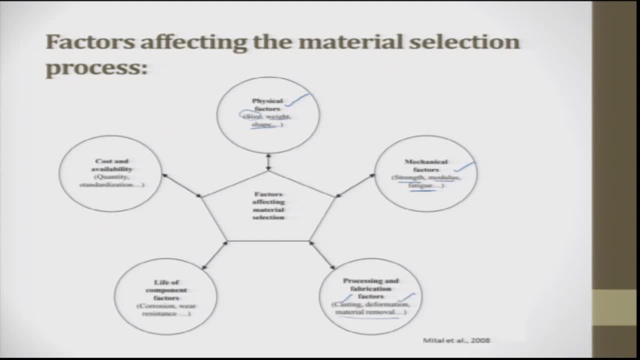 wear resistance. This is also very important. and then the cost and the availability plays a major role. So the five major factors which play a major role are physical factors, mechanical factors, processing factors, life factor, life and component factors and finally, cost. 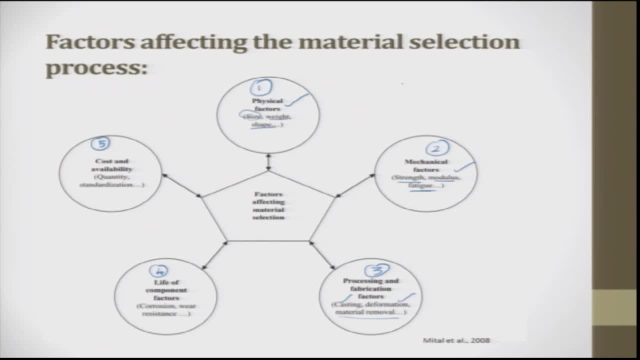 So let us take a simple example and just work for a product. I would like to develop a spoon which is used in party and my customers Customers are going to be. customers are from the age of 5 years to 70 years. 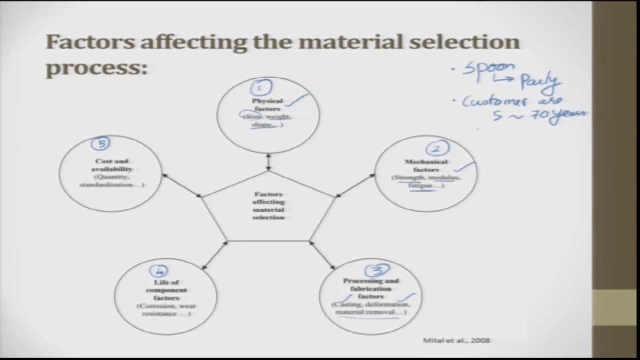 So this is what I decide. so I want to make a spoon and the cost, what I give, is going to be per spoon. I am going to give rupees 2 per spoon and I would also try to have the spoon which looks very close to that of a metal metal spoon. ok, 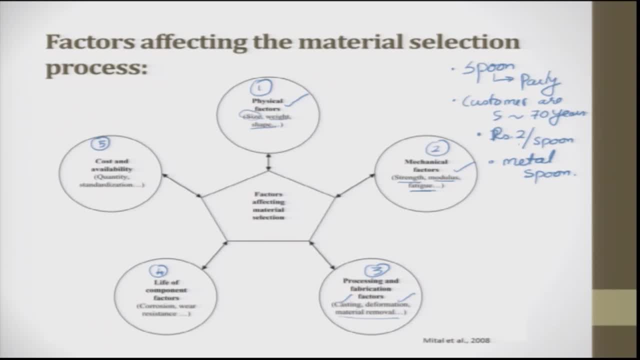 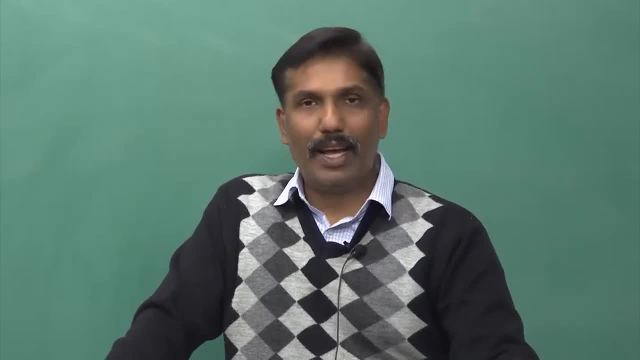 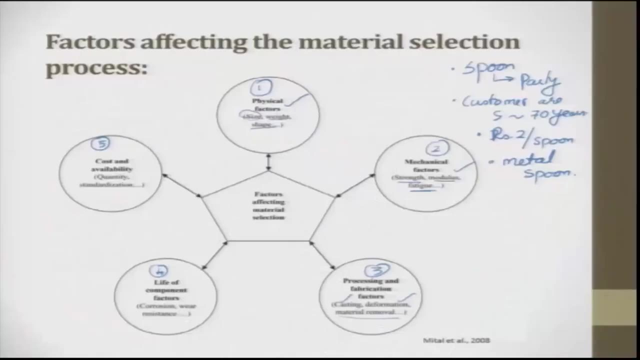 Naturally. So looking at the cost, you can quickly say that it cannot be a metal spoon. So I have to look for alternatives in ceramic spoons, or I can look for wooden spoons, or I can look for polymer spoons. ok, So then this is what I can come. 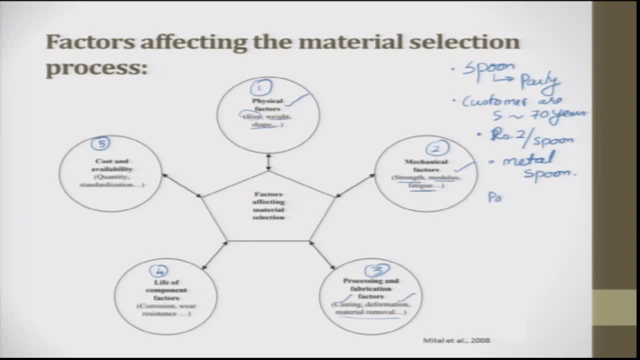 So first what I do is I try to take polymer, I try to take wood or I try to take ceramic. But what is the problem with ceramic? Ceramic is always brittle, so I try to remove this option also. So I am left with only two options. with these two options I will start working. 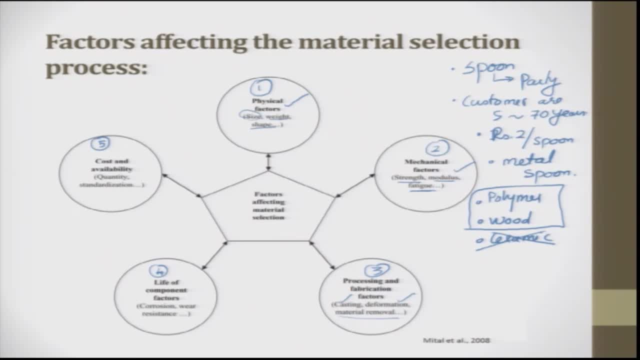 So first I would look at what should be the this polymer material or wood material, what is the maximum size I can make, what is the intricate shapes I can make in the spoon and what is the weight maximum we can give it for that spoon, and I have said it is 2 rupees. 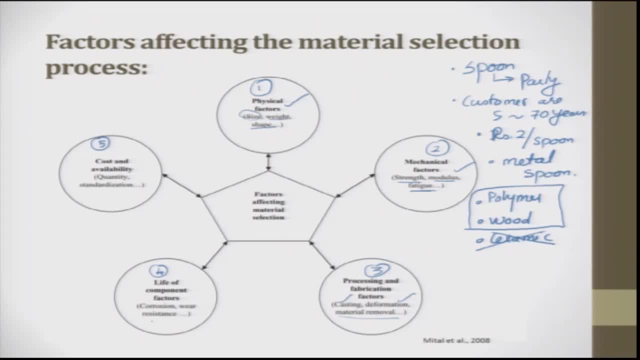 and this spoon has to be also long lasting, ok. So if it is to be long lasting, so then you can remove wood, but if it decides to have a use and throw spoon, so both these materials can be considered next. So from here I move to the next one. 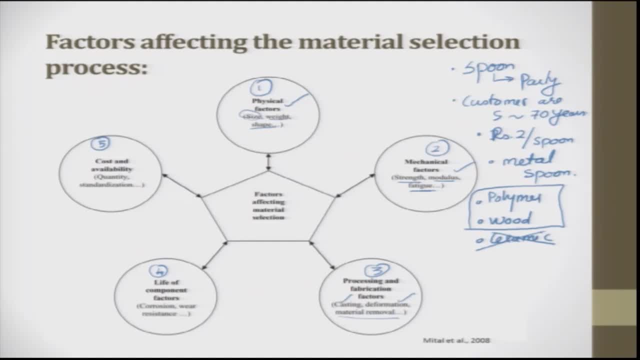 So I have chosen these two physical factors: size, shape and weight. I choose these two metal. go ahead. Next factor is I look for strength, modulus and fatigue. this is very important because when people try to eat Heavy, when that spoons are loaded very heavy, it should not deflect. 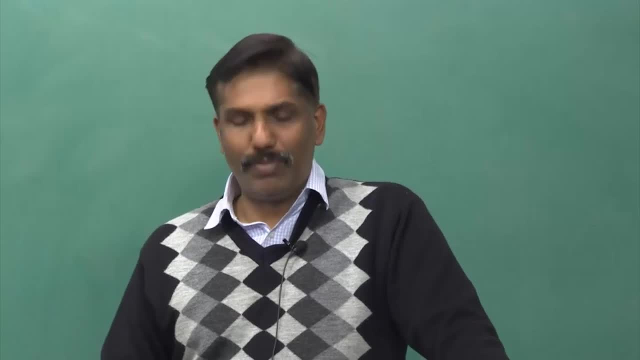 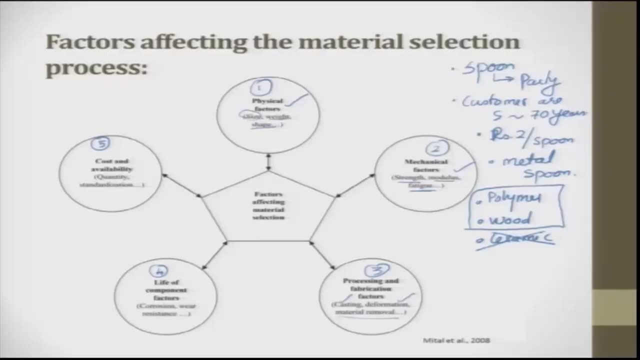 Second thing, it should not, as and when I start using in hot environment, it should not deform very fast. ok, So now what I do is I try to take these two spoons and I proceed further, but moment I said that it has to withstand heat, then the polymer spoon goes away. 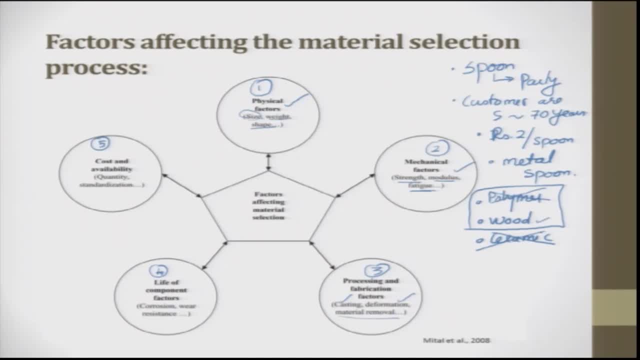 What I am left with now: wood. so now I choose wood because wood can withstand all these things. Let us talk about the next one. Now I should decide a process for making wood spoons. the processes has to be decided. So when I talk about wood, so the, the subtractive process, machining is one, the other one is: 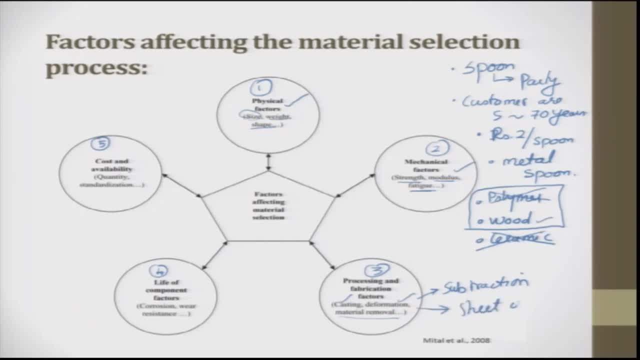 I try to take a sheet of wood and then I try to press it, try to shear it, and then I try to give a shape to it by heat. So that is just one. So that is a one, Okay, so that I get the impression of a spoon. 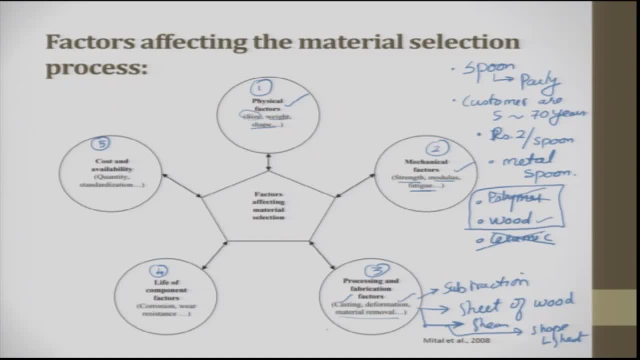 So you see, here the processing route is completely different from whatever was thought about for a wood or other things. Next I move to this factor and I say it has to have corrosion resistance and wear resistance. wood and spoon can withstand that wear resistance, of course, if it is a use and throw spoon. 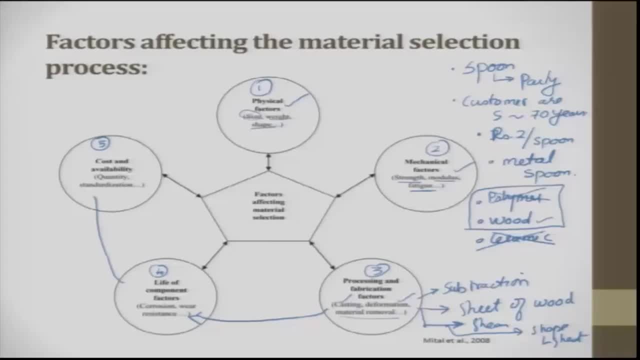 so you do not bother much, right? So then we look at cost. yes, wood is available and the standard things can be manufactured. So the cost and availability the wood fulfills it can be taken further. Suppose you decide to choose polymer as an alternative and today there is a technology. 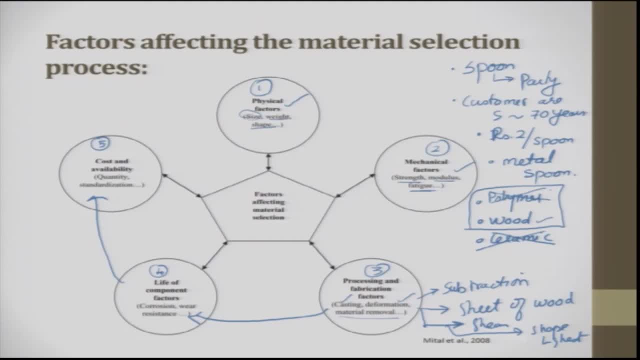 where in which you can do metallizing of polymers, which has become a very common feature. So when you look at spoons today, it looks as though it is a metal spoon, but it is a polymer spoon. So if you make that choice, the processing route is completely different. 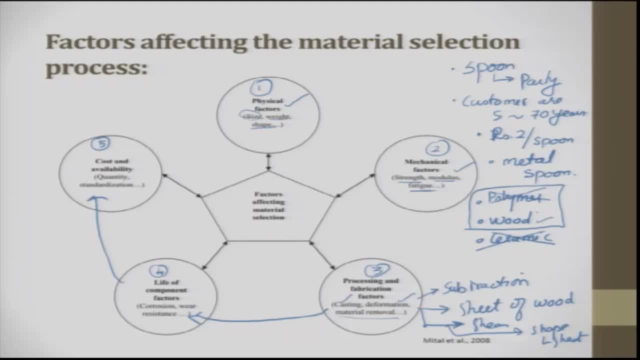 Then the life cycle is completely different. The mechanical, The mechanical properties are completely different. So, looking at the options, whatever a customer wants, you can keep start changing the material and if you make a wrong choice of material you might not be able to meet out the customers. 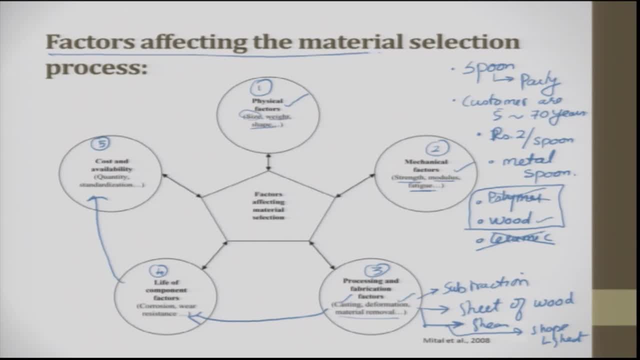 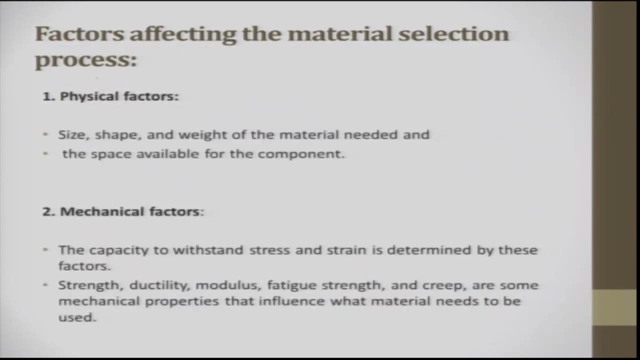 demand. ok, So this factors which affect the material selection process, all the 5 factors are very, very important. They are all linked for to the material selection factors affecting the material selection. So the physical factors, as I discussed earlier, it is size, shape, weight of the material. 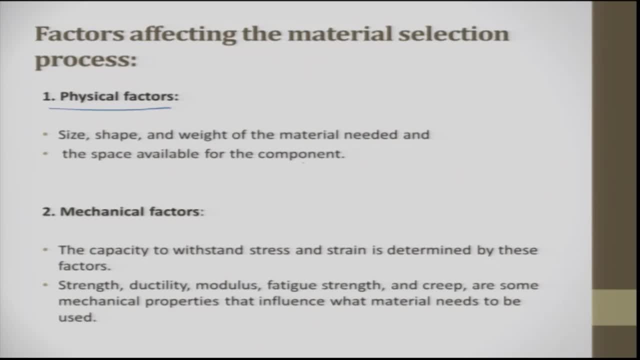 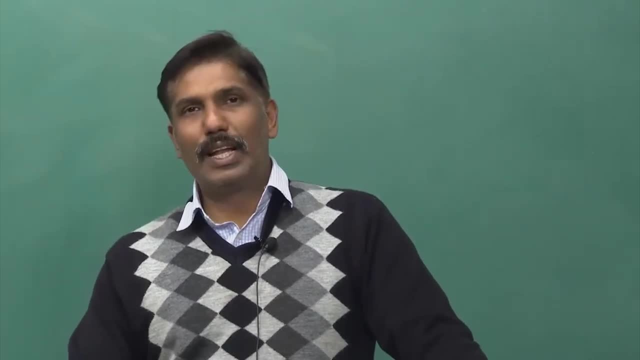 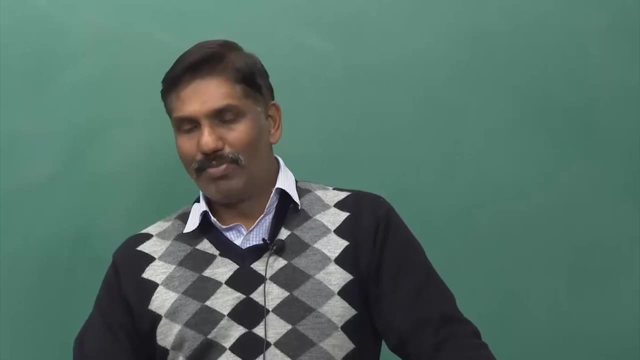 is needed. The space availability for the component is also very required is also very important. So when I talked about the example of a spoon, Spoon is a single part which is a product, but many a times in reality you will have several parts put together. forms a sub assembly. several sub assemblies put together forms a. 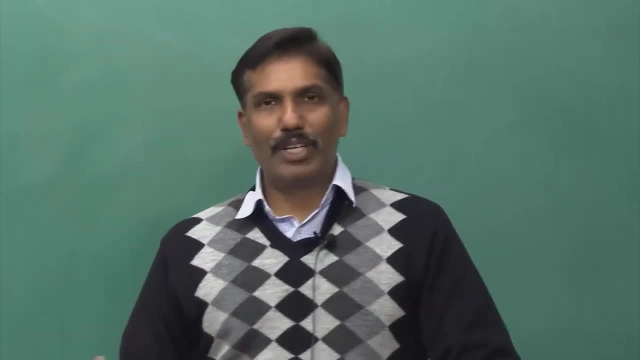 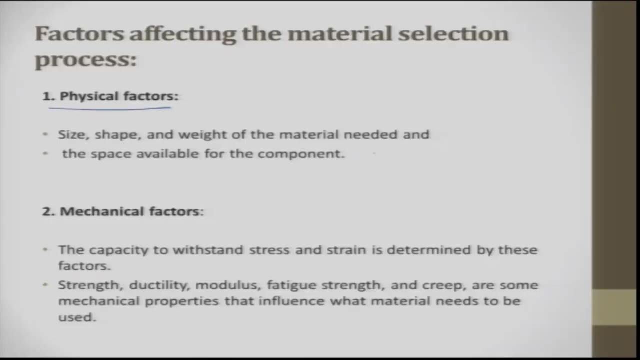 main assembly. Ok, So the shape of the space available for the component is also very important, because you might increase, for example if you choose a material with lower density. So here the volume is dictated, not the weight. For example, cotton wool: taking of a cotton wool, the volume is dictated, not the weight. 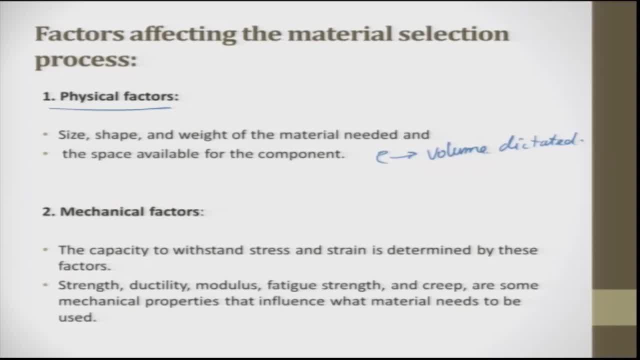 ok, So you should understand the space. So when you choose the material also, you should choose in such a way it tries to fit in the space which is available. So what are the mechanical factors? The mechanical factors which are very important are the capacity withstanding the stress strain. 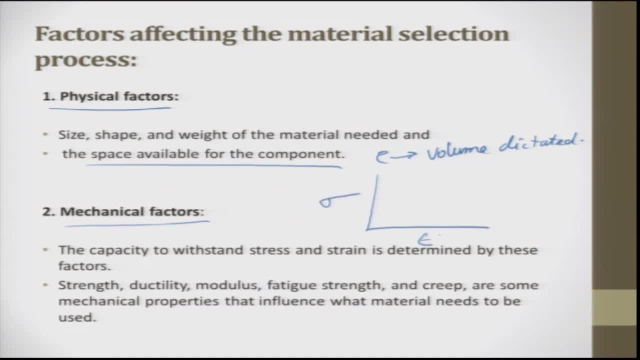 So we always go by the stress strain graph for the given material. So if it is a ductile material, it goes like this. If it is a brittle material, it goes like this: So it stands here. So we always look at what are the stress strain behavior responses for a given material. such 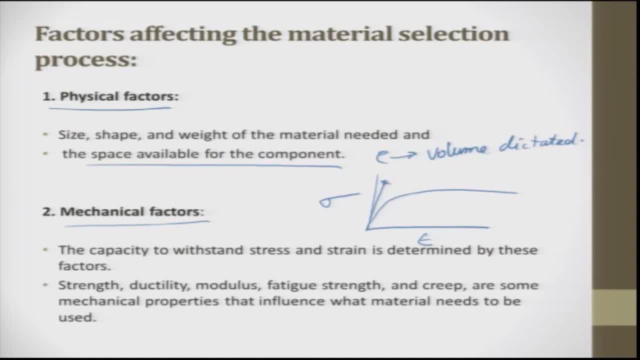 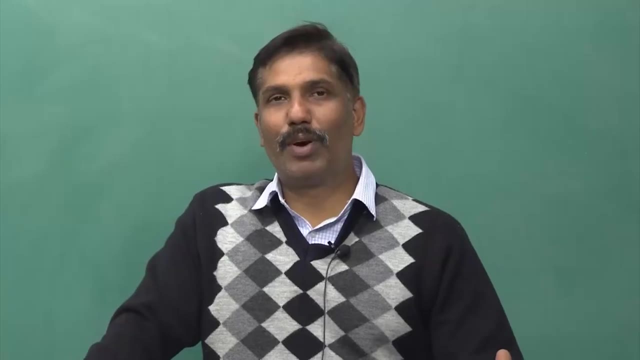 that it can meet out to the requirements. The strength, ductility, modulus, fatigue, strength, creep are some of the mechanical properties that influence what material needs to be used. Many a times it will be pretty interesting to see, all of a sudden, your flower pot, which 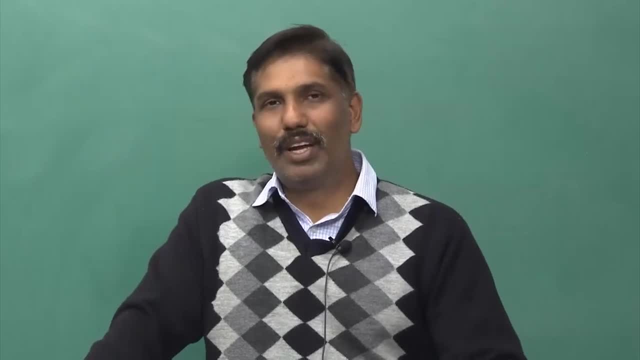 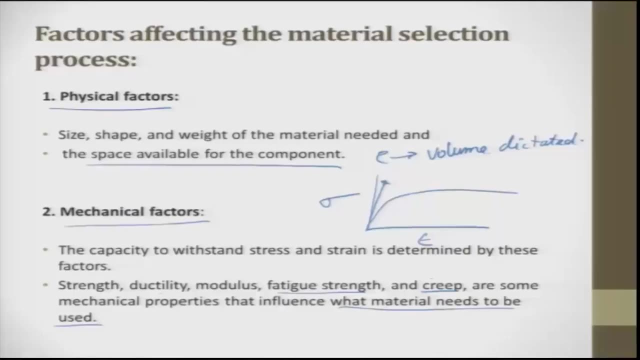 was hanging fails. So it it is. it has failed because of the creep behavior. So what happens? polymer is not having a very good creep resistance. So that is why people suggest, Whenever you put a flower pot which is hanging, please hang it using a steel rod or steel. 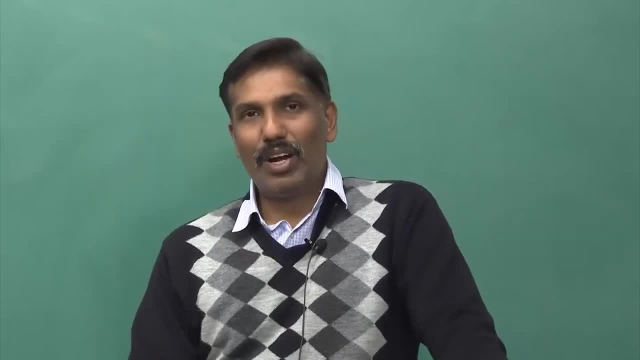 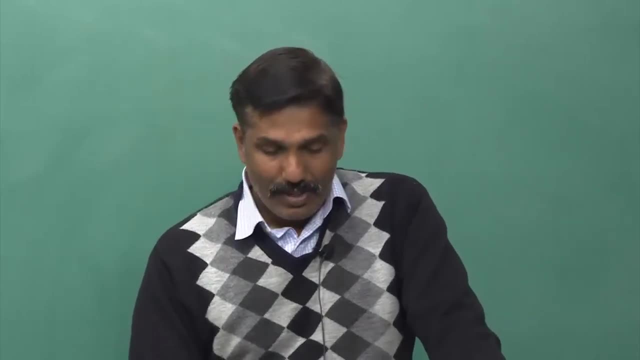 wire. But the only problem with the steel wire it it does not have the freedom of easily changing or manuring to the requirement, whereas a polymer has that facility. So when you try to choose this, you have to see those things. 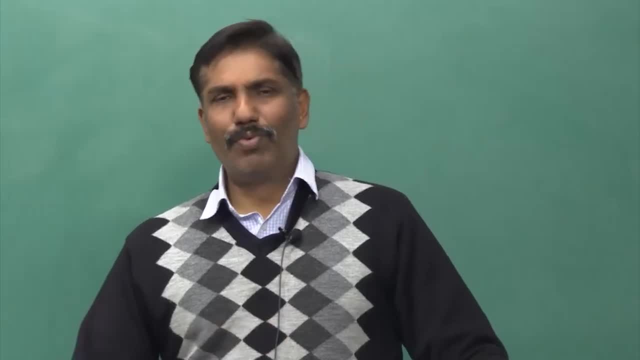 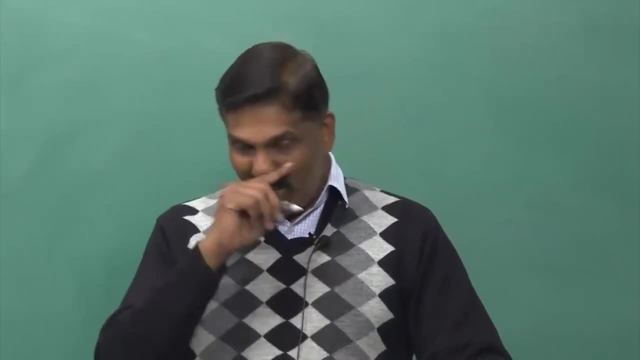 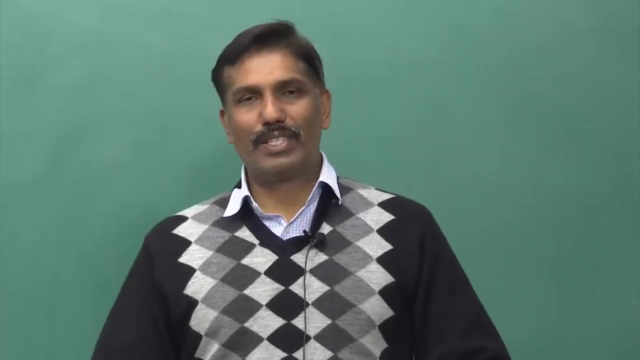 And second thing, it is also the when you see the rope which we use for drying clothes. so what happens? Polymer fails in creep behavior and it also fails when it is exposed to temperature. For example, come summer, the temperature goes to 40, 45 degrees and it is it is for 8 hours. 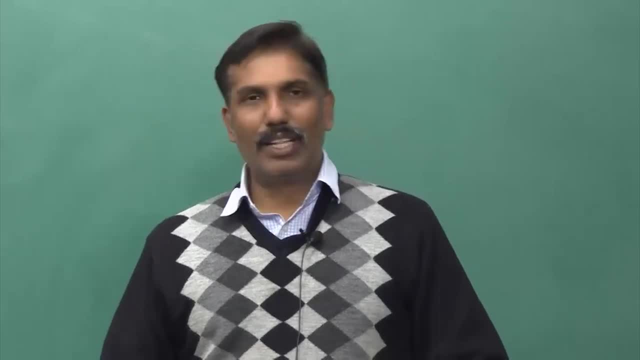 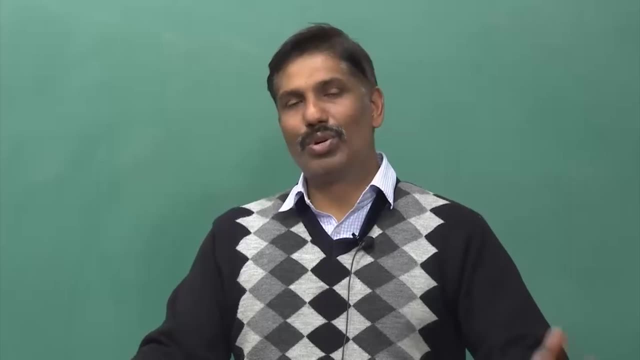 or 7 hours it constantly maintains. then immediately the polymer starts yielding, whereas a metal does not yield in those points. But when you try to choose a metal, metal always corrodes when you try to put the wet cloth on top of it. so polymer has its advantage. 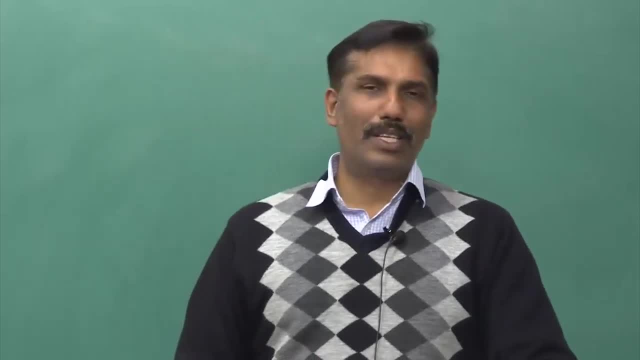 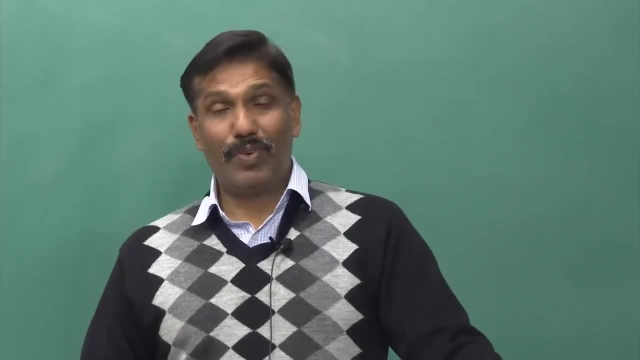 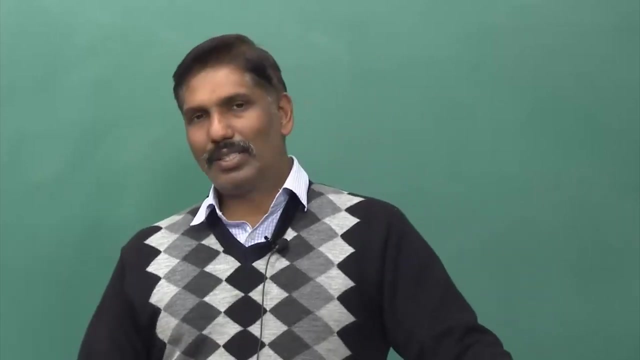 So you have to strike a balance between these two. So today, what has happened? People have started buying Polymer with a metal metal coating on top of it. it works fine. or people have started taking a metal core and a polymer tube on top of it, which is just like your wire those. 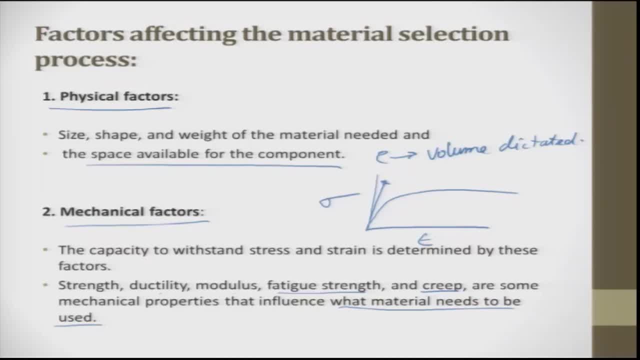 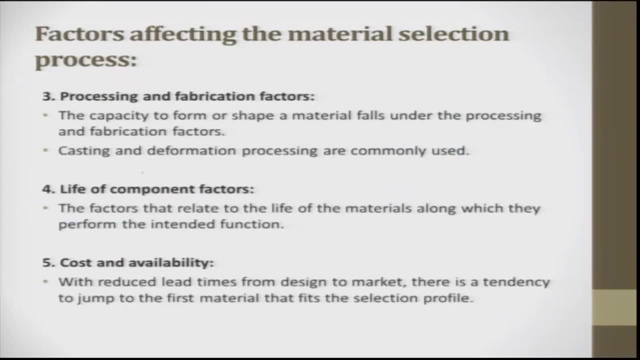 rope materials are used for drying of clothes, So mechanical factors are also very important for material selection. Next is processing. we have discussed enough. so if you want to produce any part which is very economical, We look for polymer, And then we also look for a process called as injection molding. 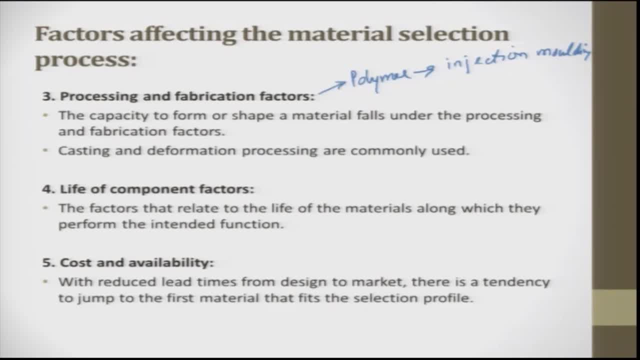 So injection molding, the cycle time is enormously less. it is round about 45 seconds. you get 10 spoons made. So injection molding is a process, whereas when you try to look at metals and if you want to do it at very economical price, so then what we do is we always go for metal. 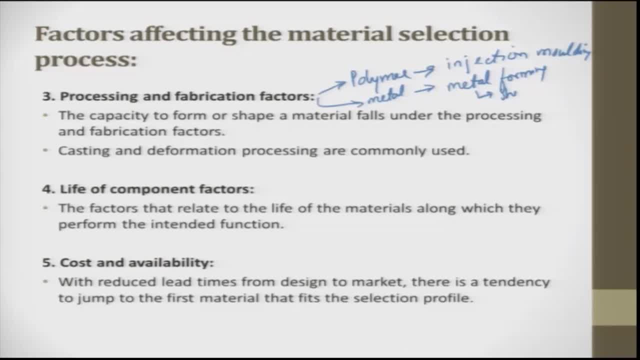 forming. So that means to say sheet metal pieces are used, sheet metal, sheet metal are used so that it can start making it. So casting and deformation process are constant volume process where in which the starting material and the ending- if you sum up, the end- a products, it will be almost the same. 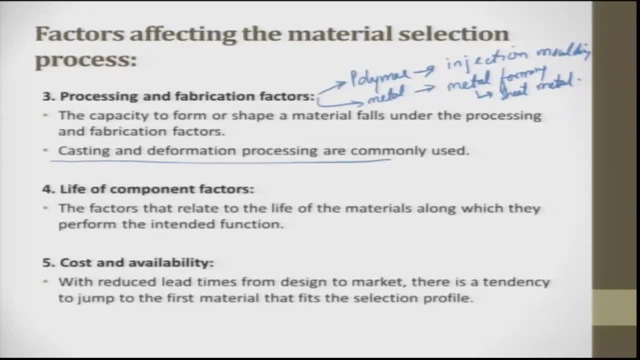 it is a constant volume process Here it is not thought of. this process is not thought of for a mass production. mass production where the product cost is economical, the life of the component place an important factor and the cost and availability also plays a very, very important role in choosing. 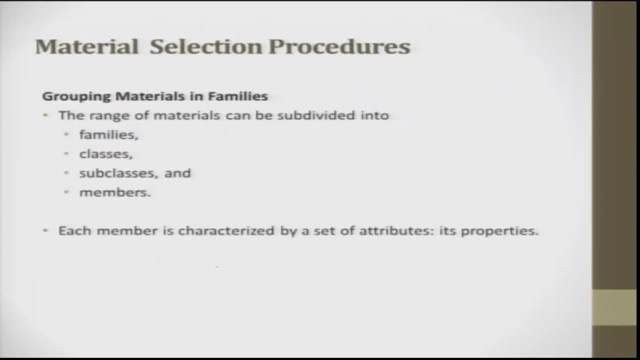 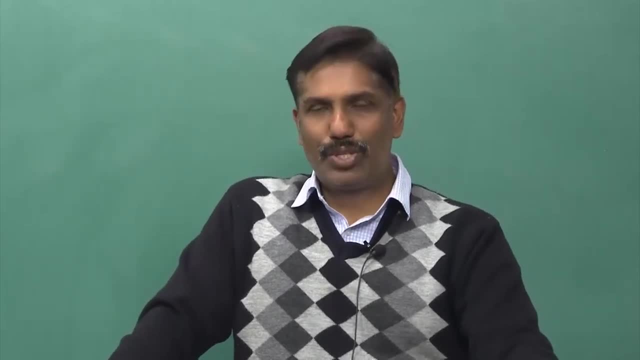 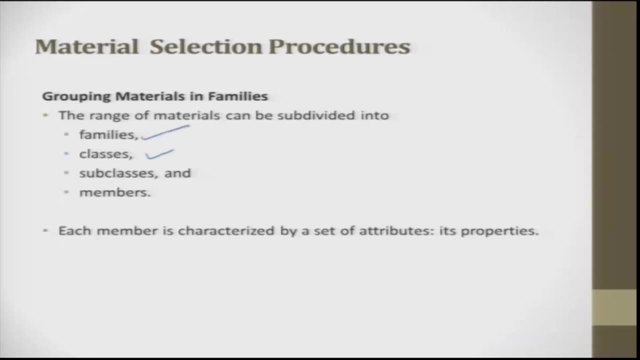 the material, The like in in biology, botany and in zoology, we have a, a, a toxonomy followed. So here in material selection also we follow a toxonomy, which we talk about family, class, subclass and members. ok, So a range of materials can be subdivided into families, families. 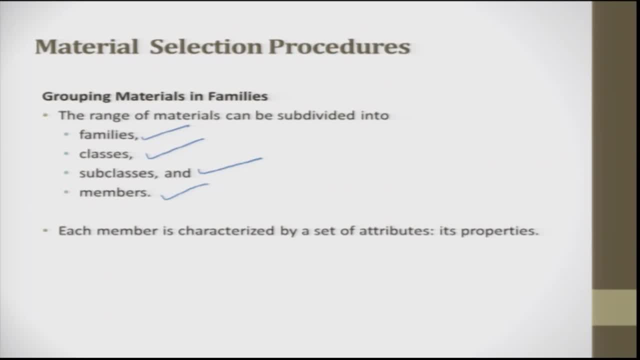 further will be divided into classes. classes will be further divided into subclass and subclass will be divided into members. So why is it done? Suppose, if you are able to, you are able to identify the customer need and you are looking for a material for your 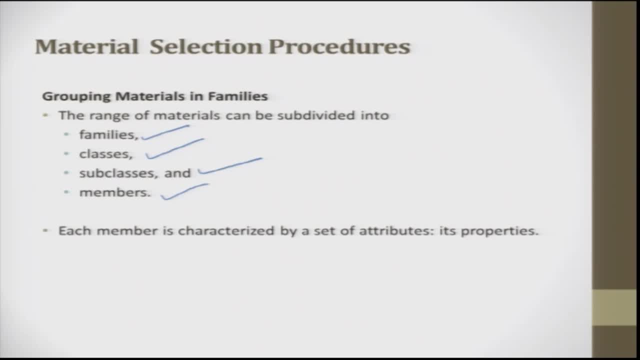 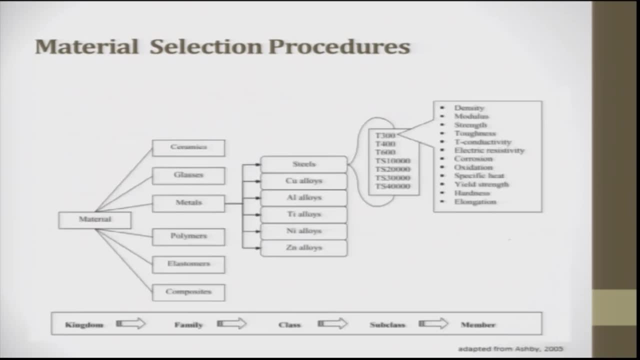 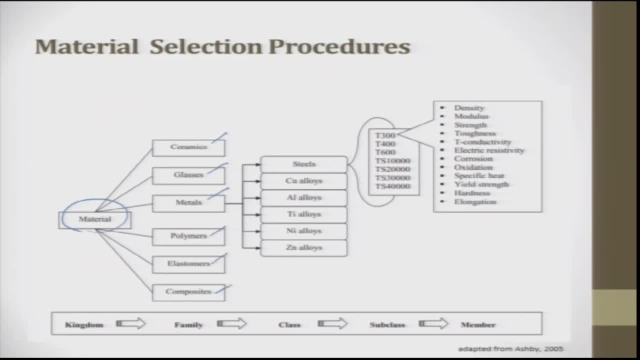 glass, glass, glass metal, polymer, elastomer and composite. These are all family is attached to the kingdom called material. When I choose a metal, it is basically ferrous and non-ferrous, So it is a steel, and then you have non-ferrous materials, So it is. 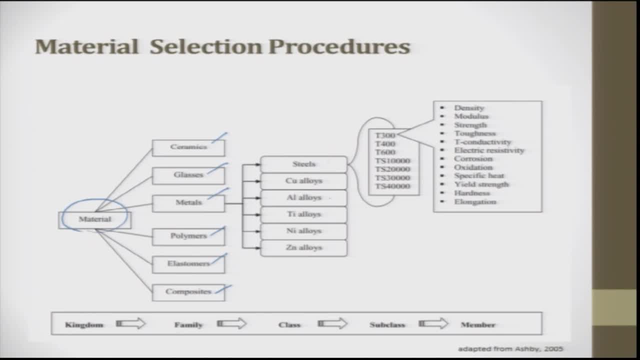 steel and all the non-ferrous- copper alloy, aluminium alloy, titanium alloy, nickel alloy and zinc alloy. So all these material are are um having strength which are lower than steel, And they are also that density is also less as compared to that of steel. 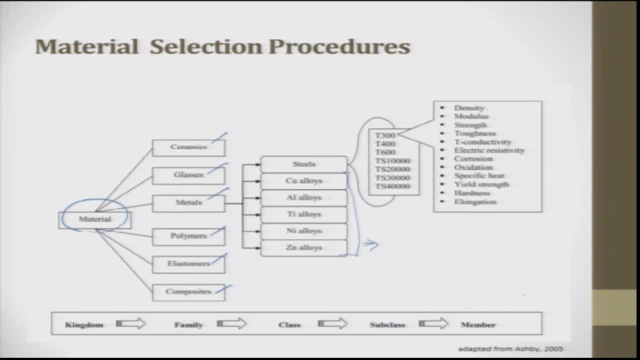 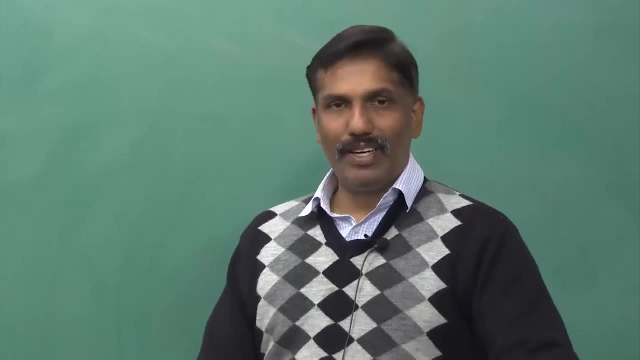 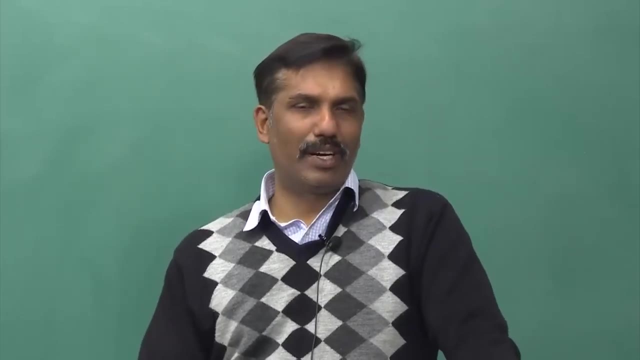 If you are looking for primary application, that means to say primary application as weight taking, ok, primary structure, load bearing. So then it is better to have a steel one. Suppose you are looking at some structure where in which it is a secondary structure, not of load, but it needs to have lot of heat conduction. then we go for copper. 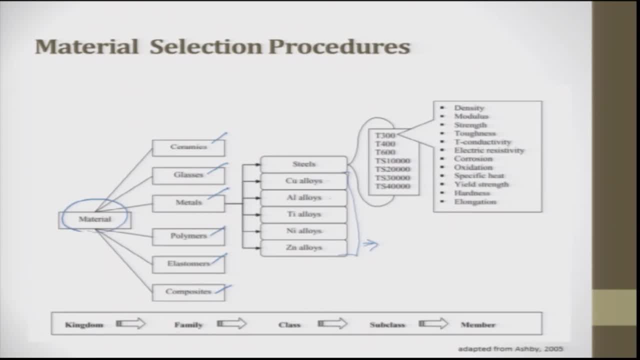 If it is going to be secondary structure which has to be light and no heat taking, you can think of aluminium. All the PACE vehicles. they try to use titanium alloy and nickel alloys because they are light in weight, they have very high strength properties and these by combination with several alloys. 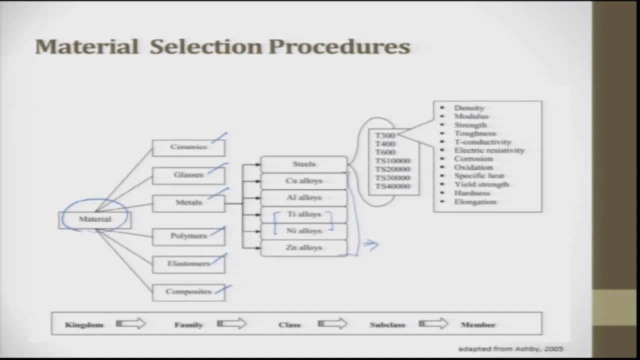 show different performance when you put in even vacuum or when you put at very low temperatures, So when you again. so this falls in the class. So first is kingdom family, metal family, and then from the family we get into, fall in the classes. 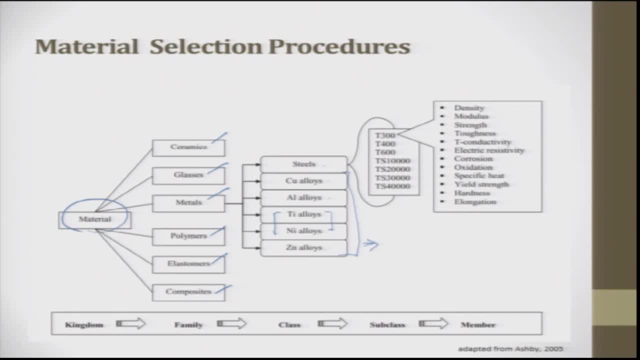 So this steel is again sub classified into two, So T 300, T 400, 600, whatever it is, 10,000, 20,000, TS 10,000, TS 20,000, 30,000, 40,000.. 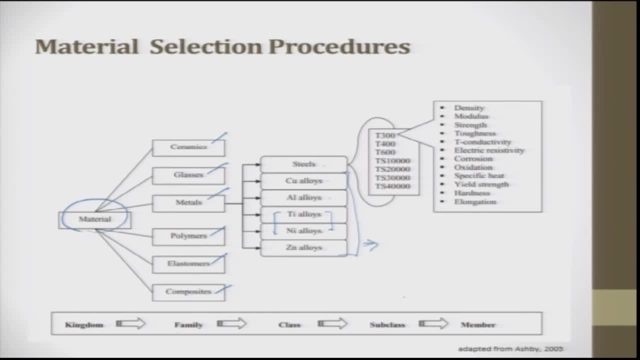 So this, these nomenclature basically tries to talk about the copper which is present in the carbon, which is present in the steel, and also some properties. So this is a subclass of this is a class. this is a subclass, then what are then you?